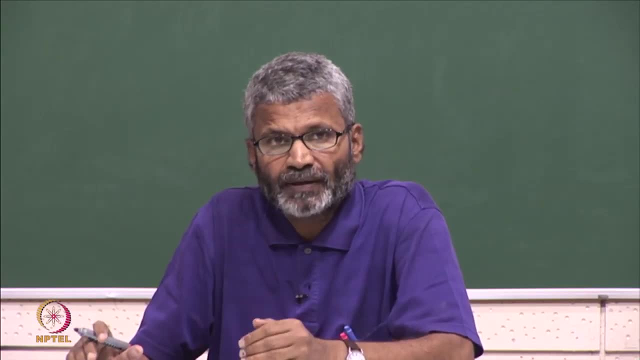 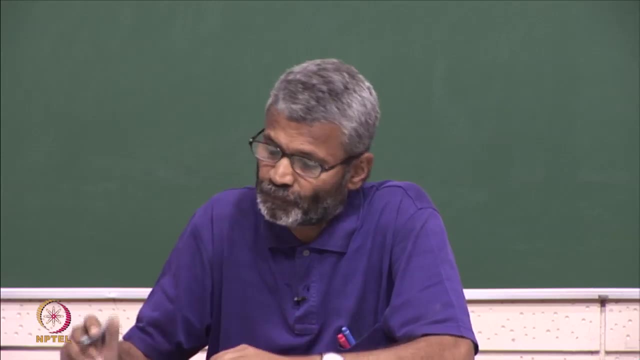 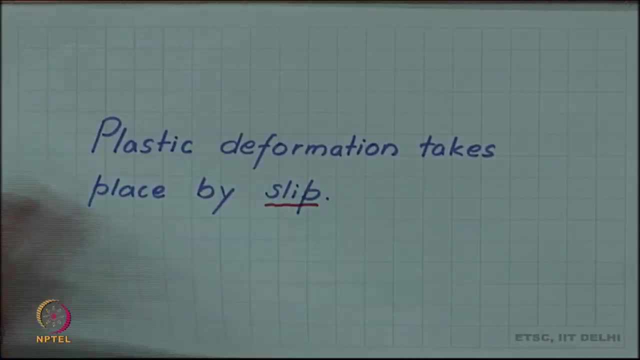 change. the external shape changes, but internally, the unit cell does not deform. the unit cell remains the same. the crystal structure remains the same. So to explain that the plastic deformation was understood To take place by slip, and by slip we meant that one part of the crystal slides over the 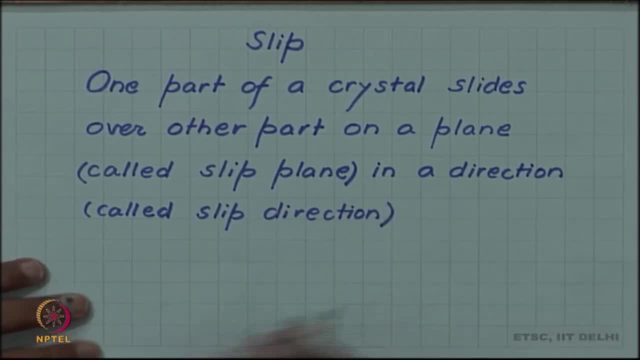 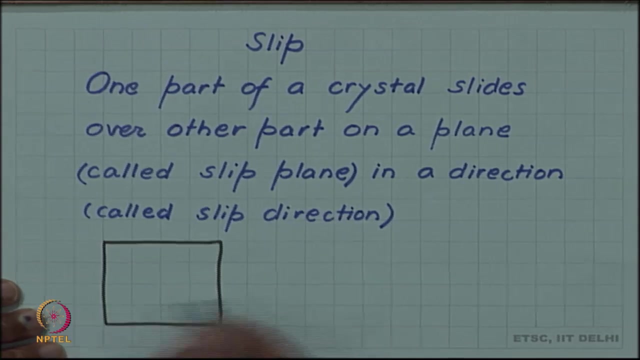 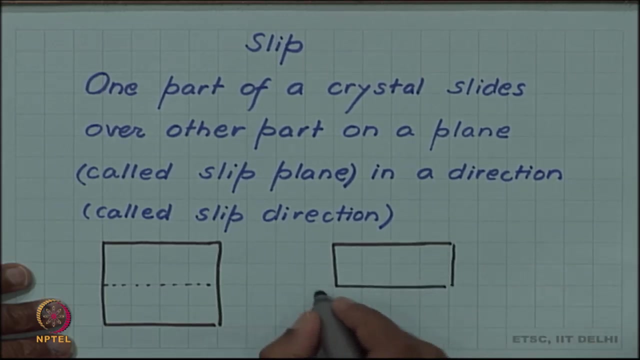 other part on a plane called slip plane in a direction called slip direction. Recall that we had something like. so we say that if we have a block of material and if this is deforming, one way of deforming is that on a plane like this, if the upper half slides with respect to the lower half, then we have 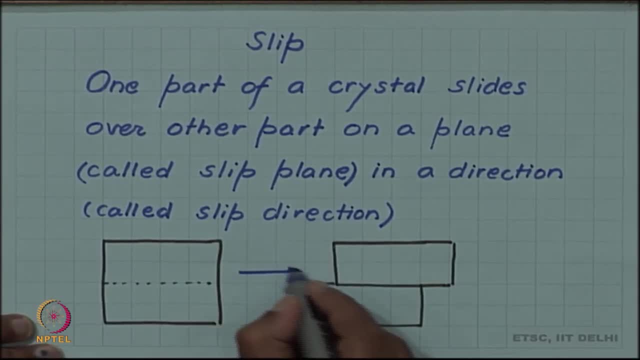 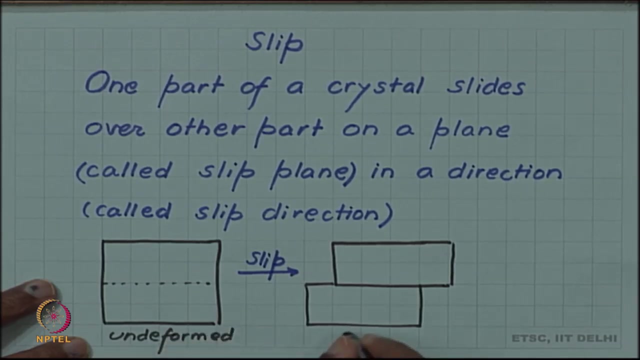 obtained deformation. So this is what we are calling slip. this was undeformed, this is deformed and we will call this plane the slip plane. So this plane is the slip plane and this direction will be the slip direction. So this is the basic mechanism we are accepting for plastic deformation. Now the question: 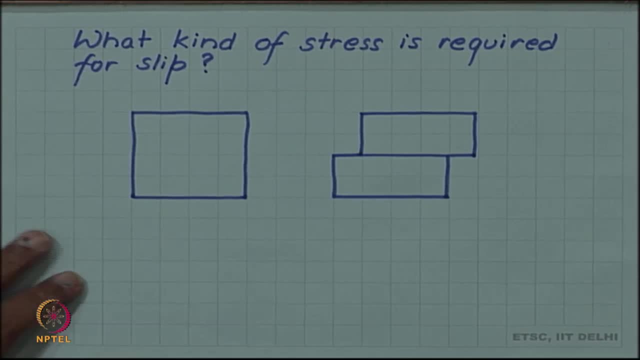 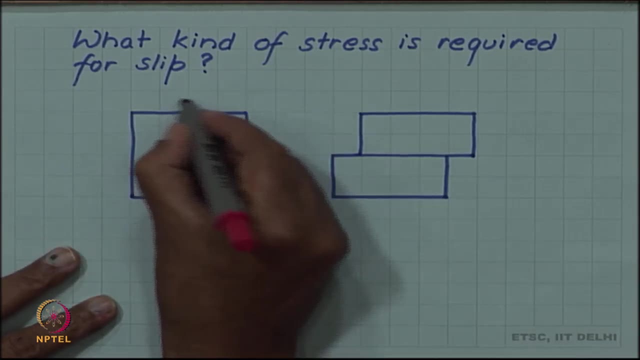 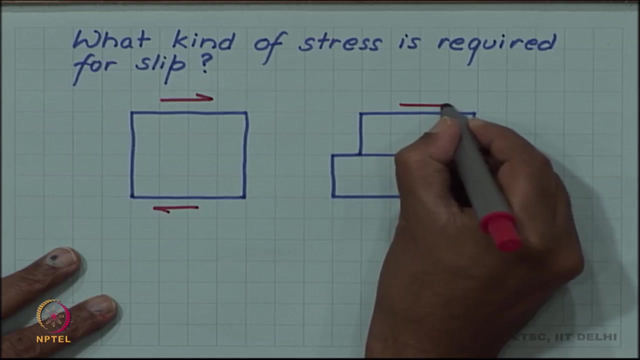 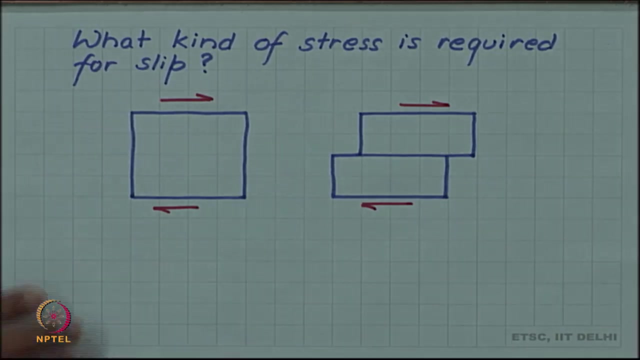 is what kind of a stress will be required? if this is the basic mechanism, what kind of a stress will cause this deformation to happen? and we can see that for slip to happen, the required stress will be a shear stress. You have to apply a shear stress on the slip plane in the slip direction for slip to happen. 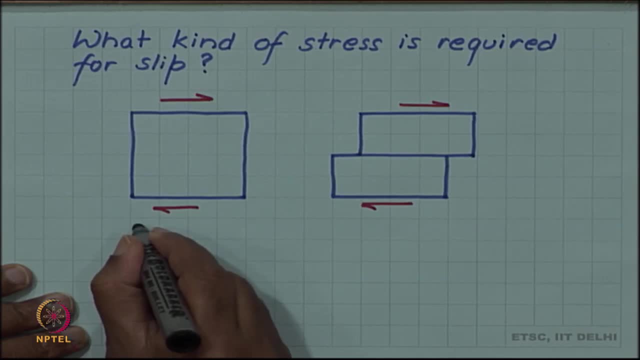 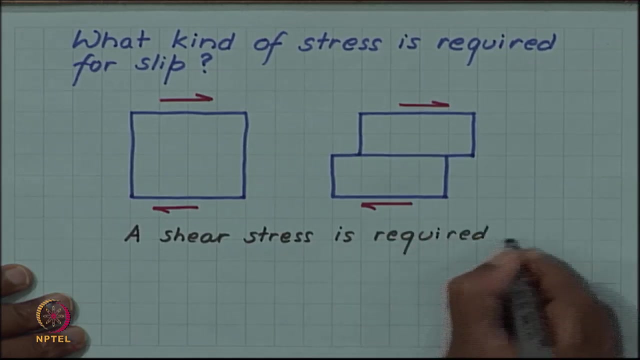 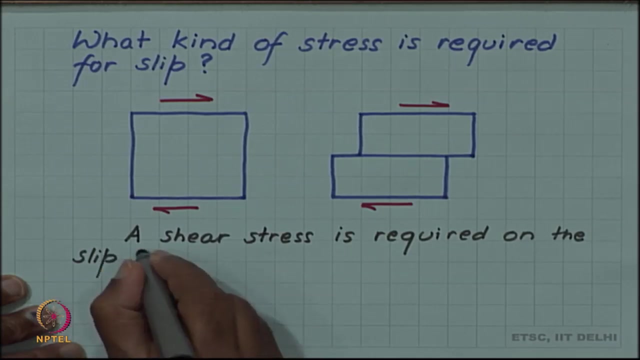 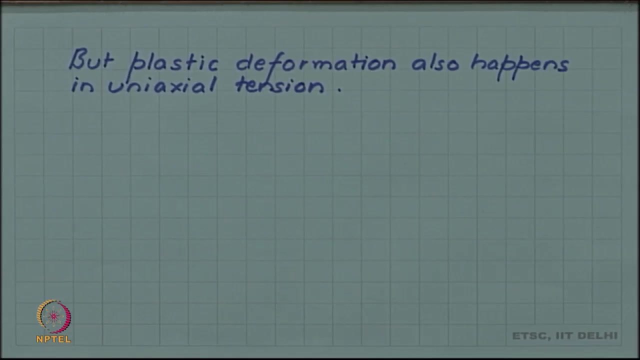 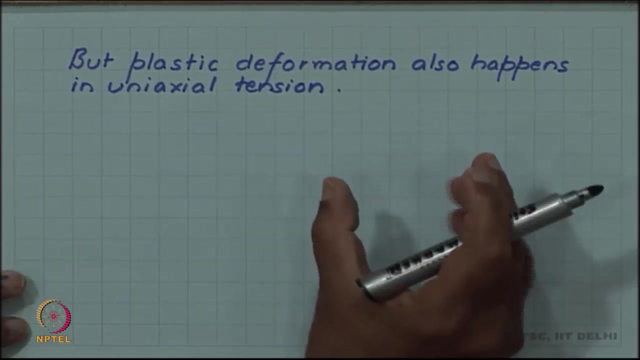 So the shear stress is required. This shear stress is required on the slip plane, in the slip direction. But then we have also seen that plastic deformation also happens in uniaxial tension. in the beginning of this chapter We discussed uniaxial tensile test as an important test for deriving mechanical behavior of the 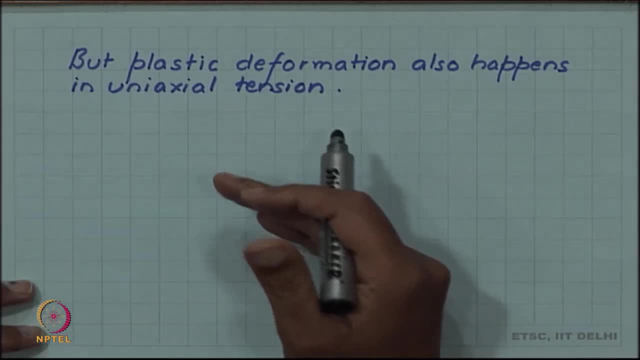 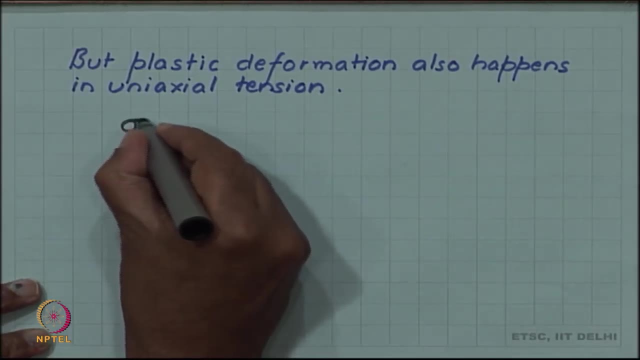 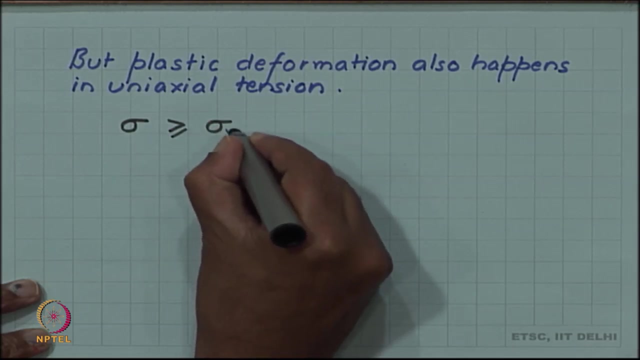 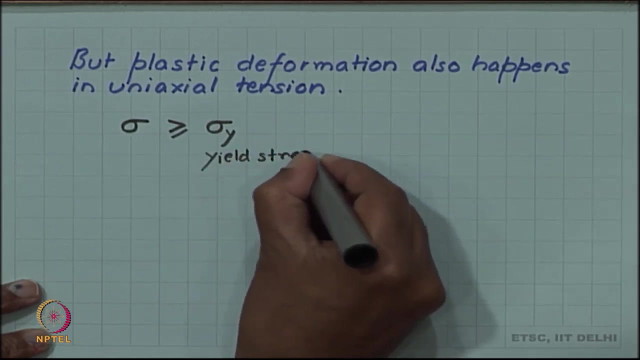 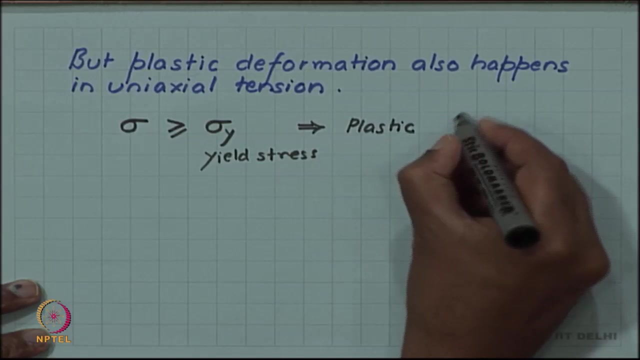 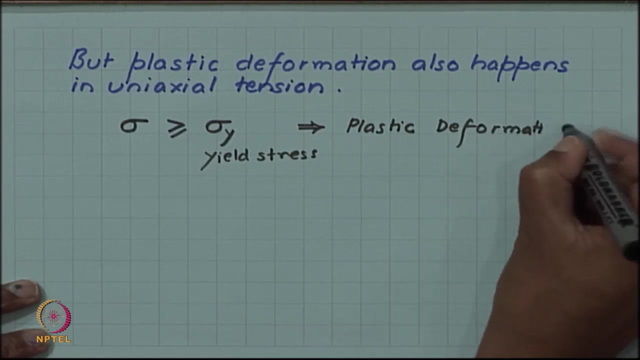 material. and there we saw that initially, although the material deforms elastically, when the tensile stress reaches a critical value of stress called the yield stress, sigma y, which is the yield stress, Then plastic deformation happens in uniaxial tension. But then this suggests that if slip is the mechanism, then this uniaxial tension should. 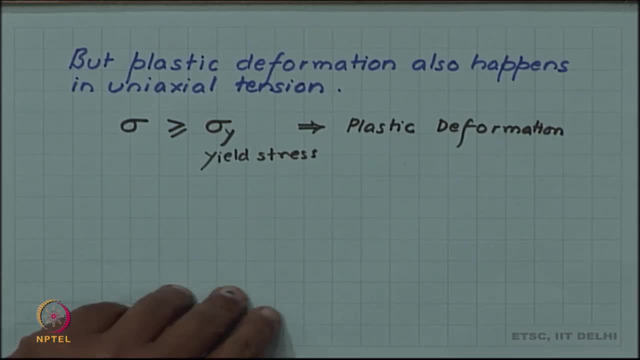 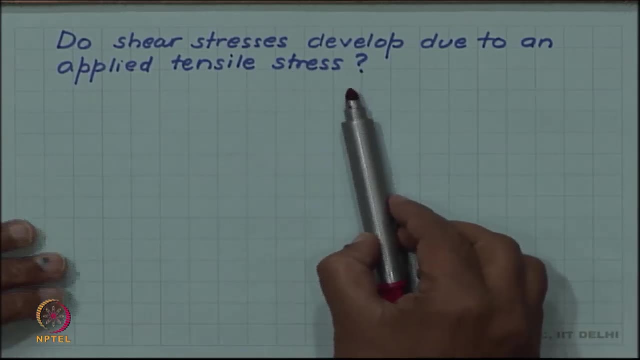 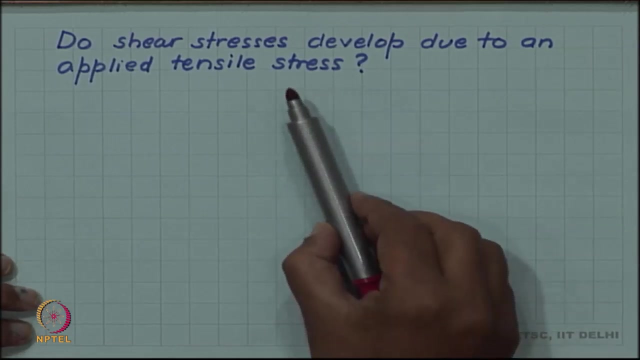 be leading to shear stress on the slip plane in the slip direction. We have a question that: do shear stresses develop due to an applied tensile stress? because if slip is the mechanism of plastic deformation and tensile stress is causing the plastic deformation, So that tensile stress should be capable of generating shear stress on the slip plane. 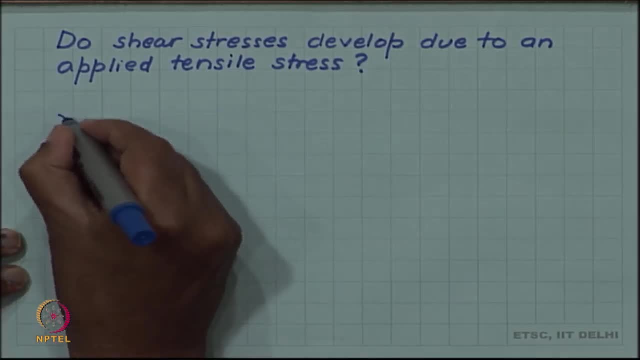 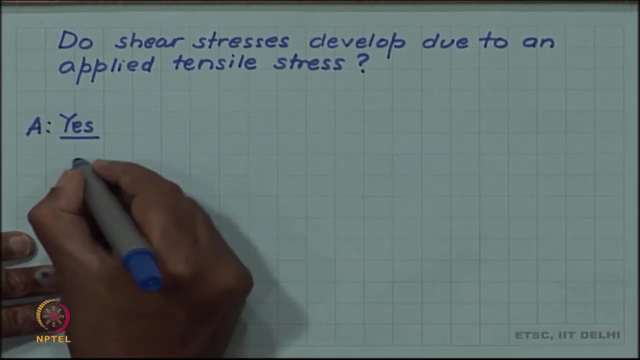 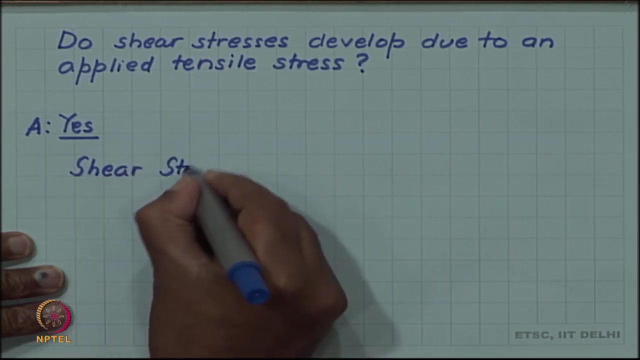 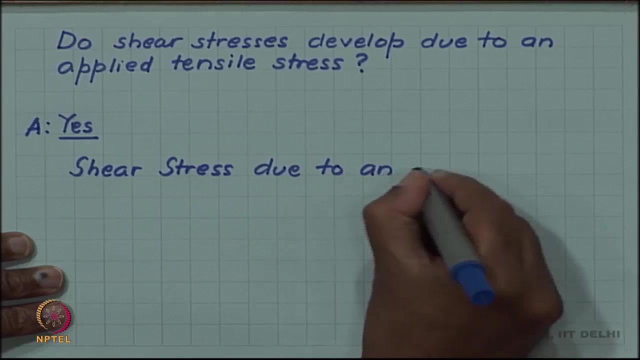 in the slip direction. So the answer to this question is yes And Yes, Yes. So let us write the measure: load rejoicing flow ох and the stress generated- the shear stress to an applied tensile stress. And the stress generated- the shear stress- due to an applied tensile stress. 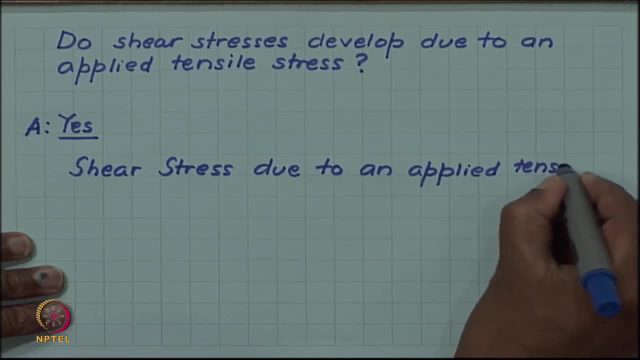 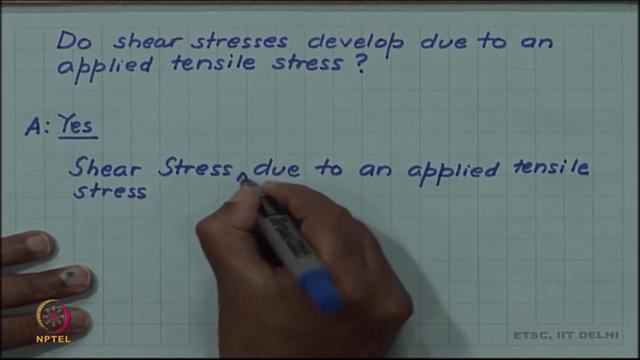 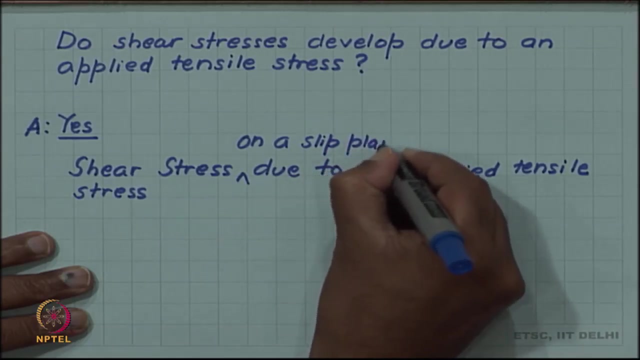 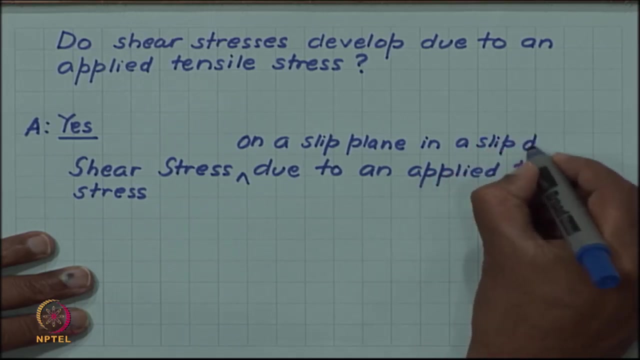 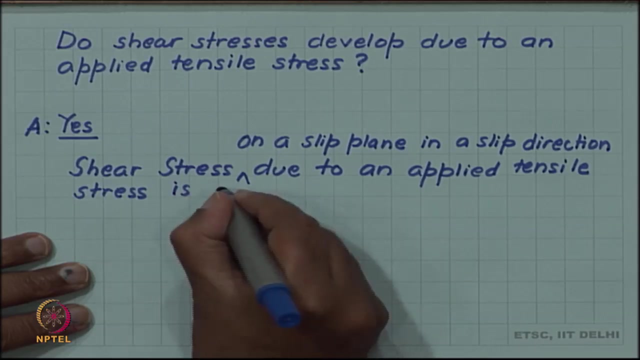 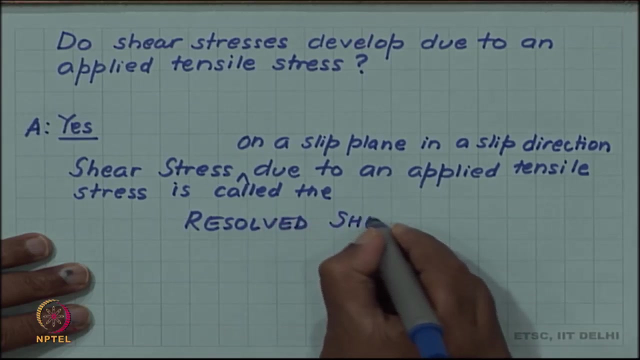 When the stress being generated- seiеле stress As heading of the surf, shear stress on a slip plane in a slip direction due to an applied tensile stress is called the resolved shear stress. Sometimes we will abbreviate it to RSS and sometimes we will use the symbol. 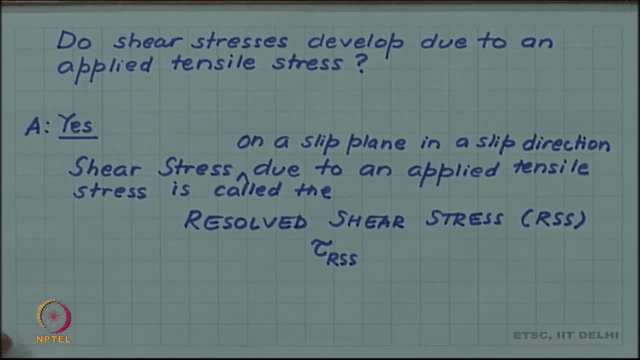 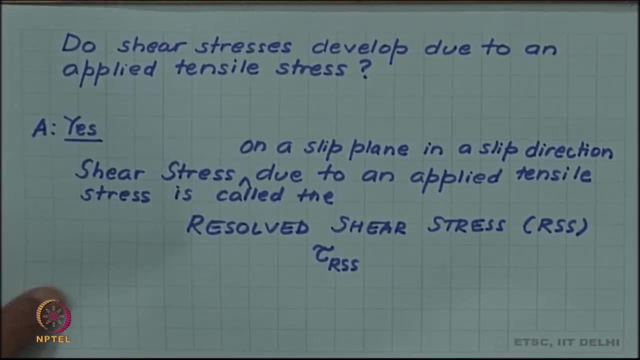 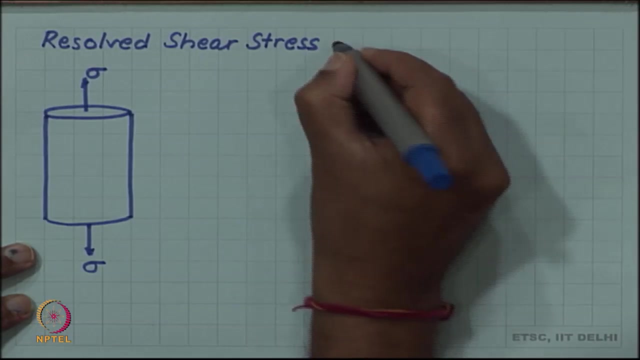 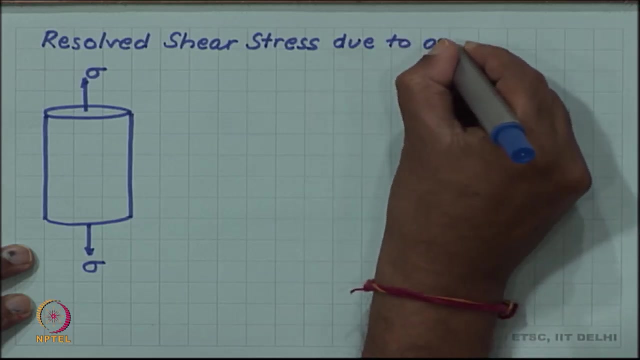 So for shear stress and put RSS as subscript. so this is called the resolved shear stress. So let us now try to find that, given applied tensile stress, how much resolved shear stress will be generated. So resolved shear stress due to an applied tensile stress is called the resolved shear. 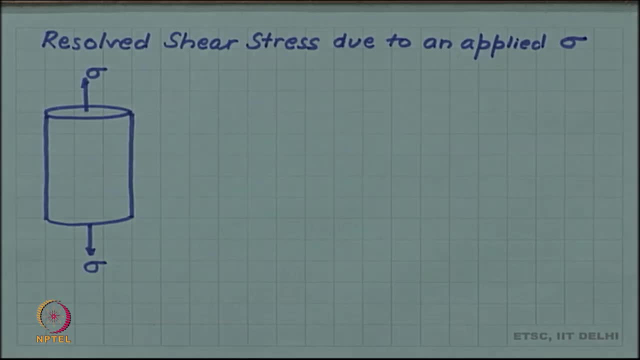 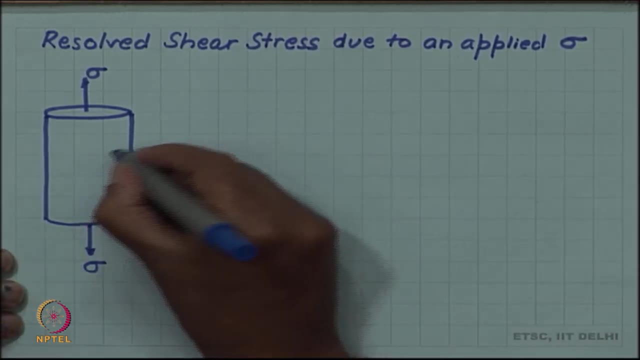 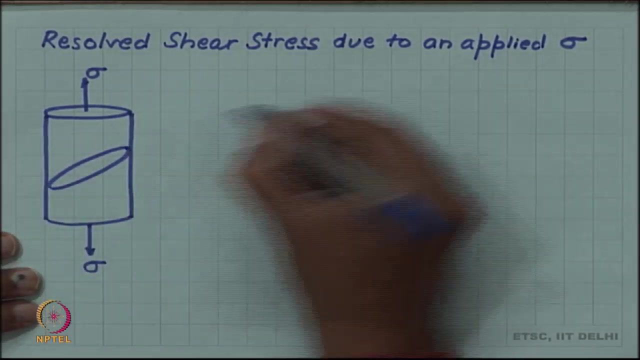 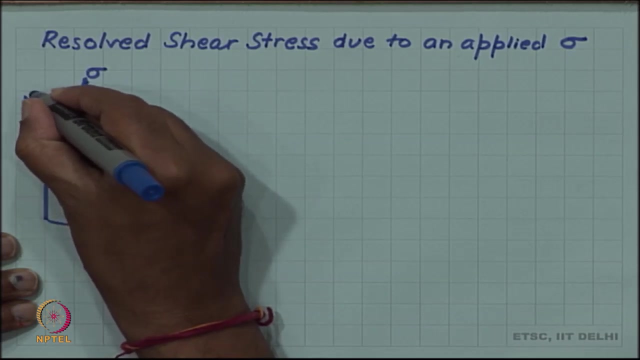 stress, Tensile stress sigma, as shown here. for this, first we have to identify the slip plane. So let us include a slip plane in this. So I am including an inclined slip plane such that the normal to the slip plane normal. 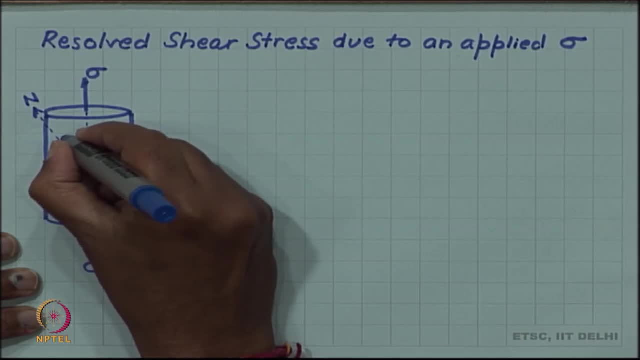 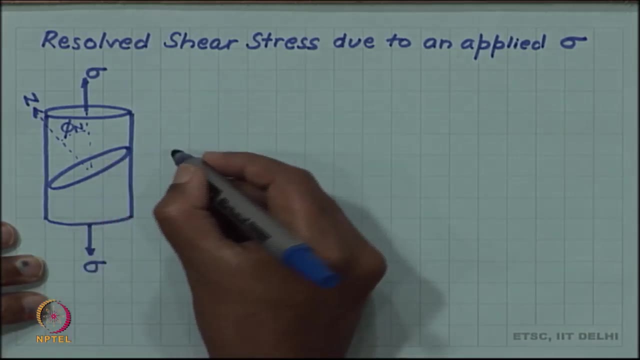 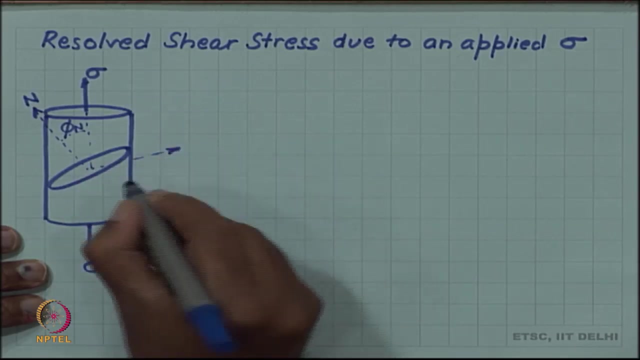 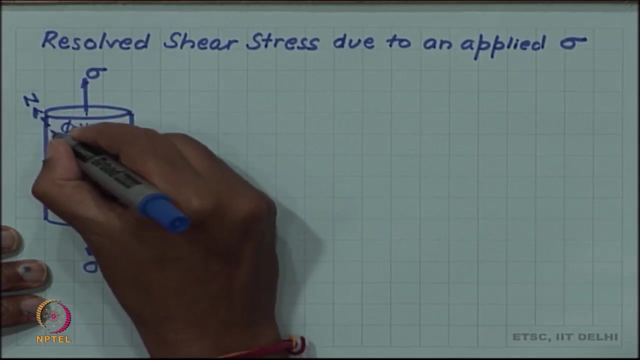 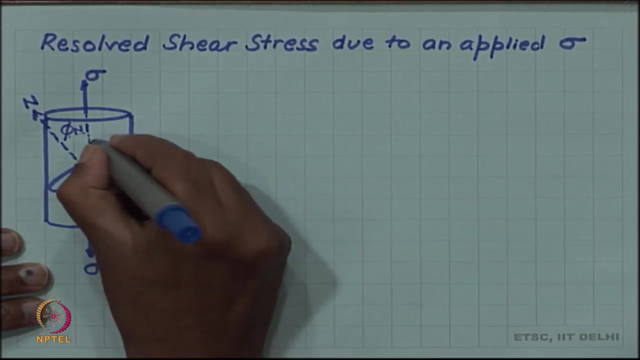 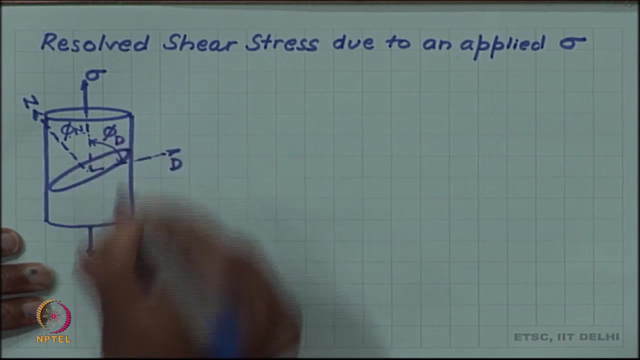 end to the slip plane makes an angle, So this is the angle phi n. and let us say d is the slip direction and the tensile stress makes an angle phi d. So this is the angle phi n. This is the angle phi n with theria top, with the slip direction. 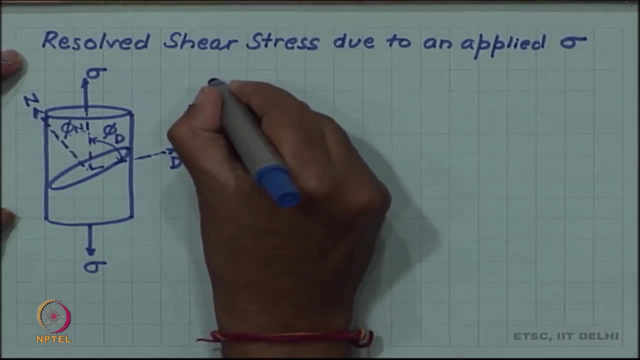 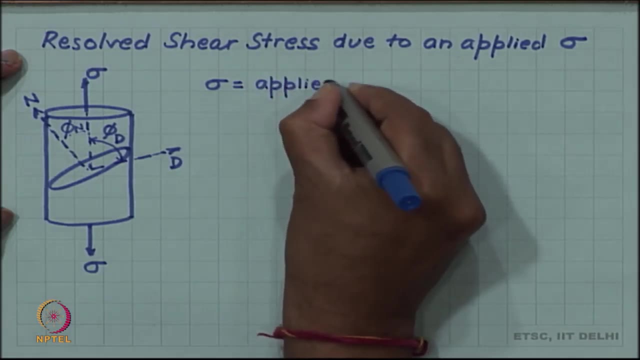 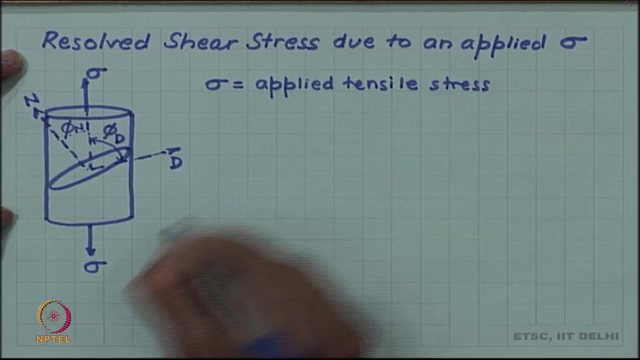 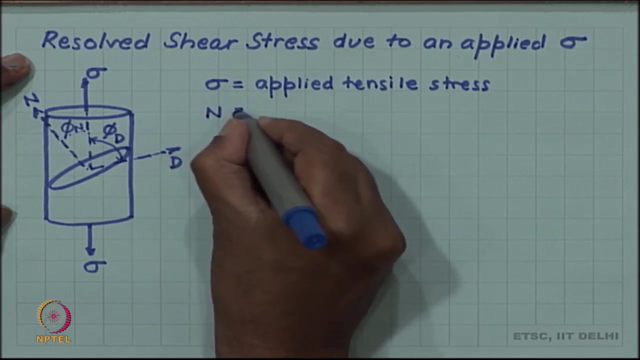 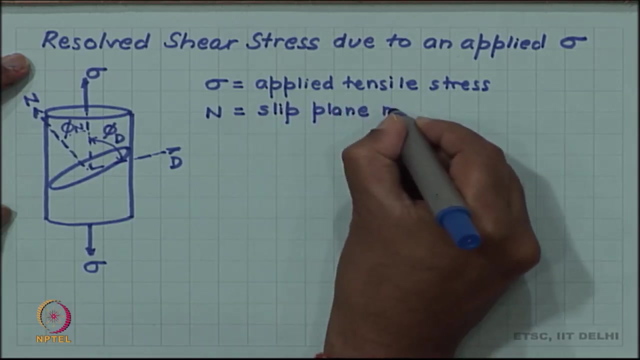 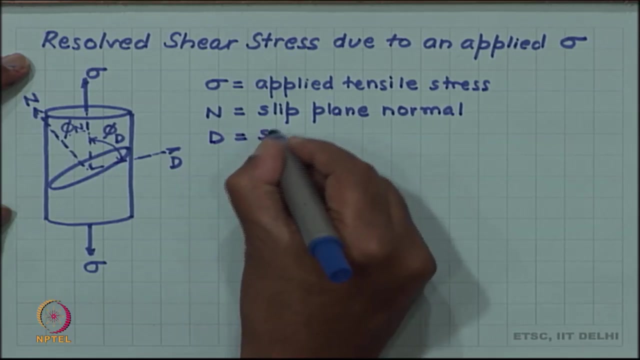 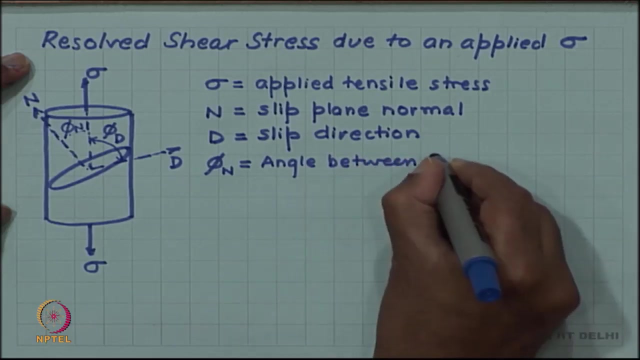 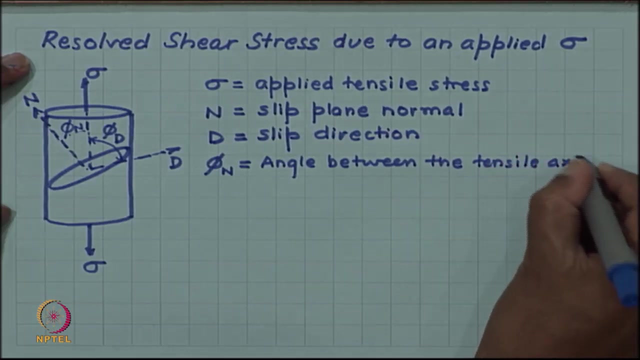 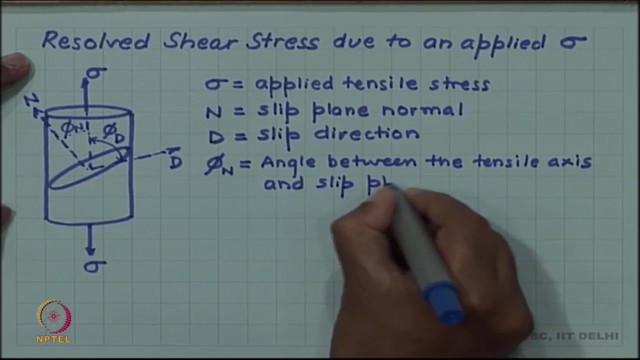 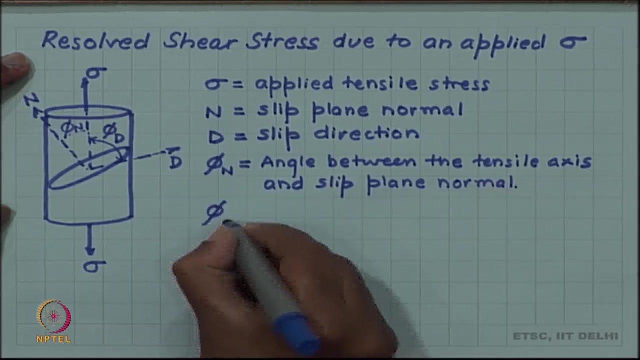 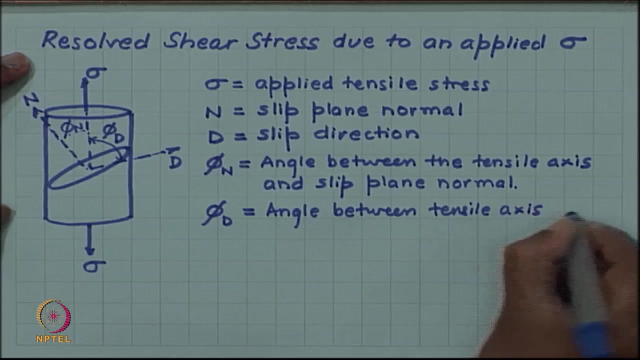 So let us write now our variable. so sigma is the applied tensile stress. Okay, n is slip plane. normal d is slip direction. phi n is angle between the tensile axis and slip plane. normal phi d is the angle between axis and slip direction. 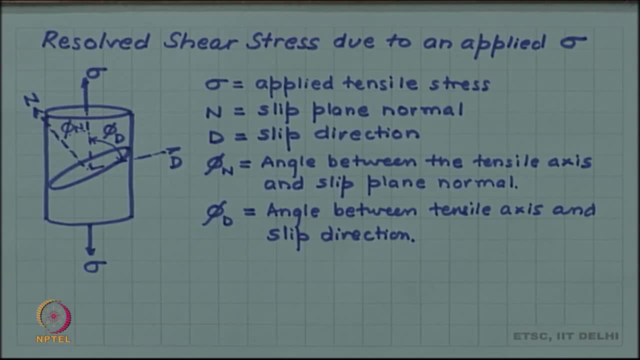 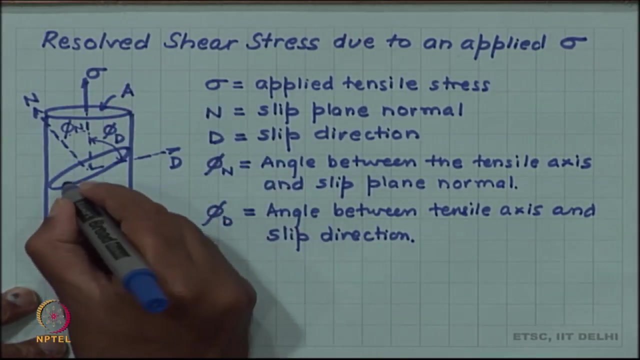 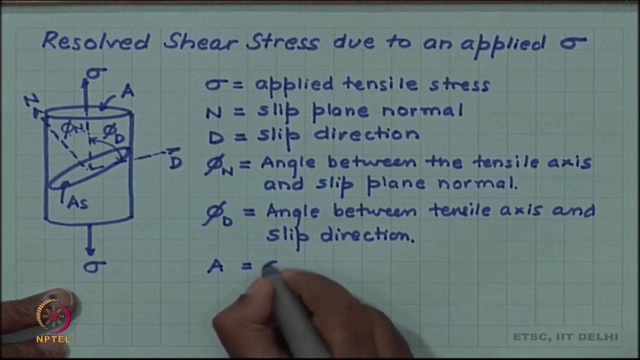 So with these variables we can try to find what is the resolved shear stress tow. Let us also define- we will need this- the cross sectional area A and the area of the slip plane A s. So A is cross sectional area of the specimen. 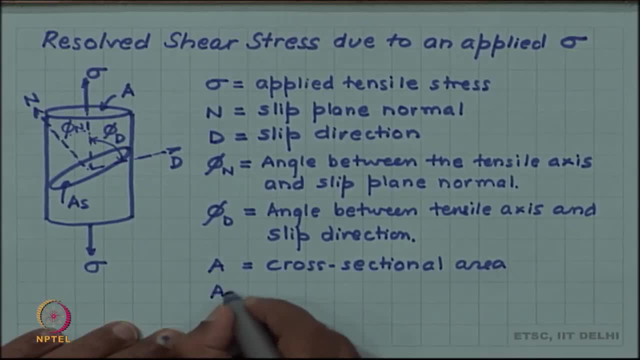 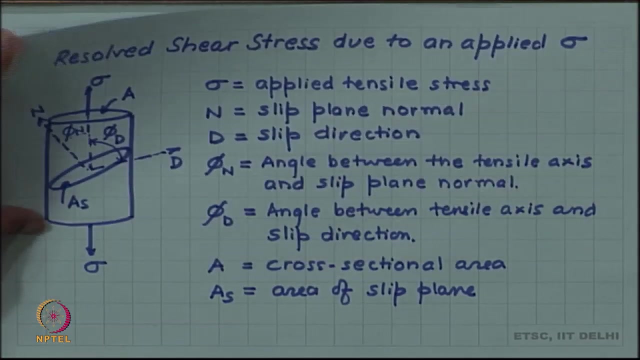 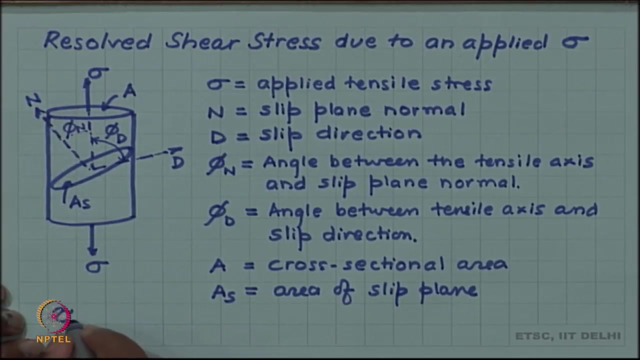 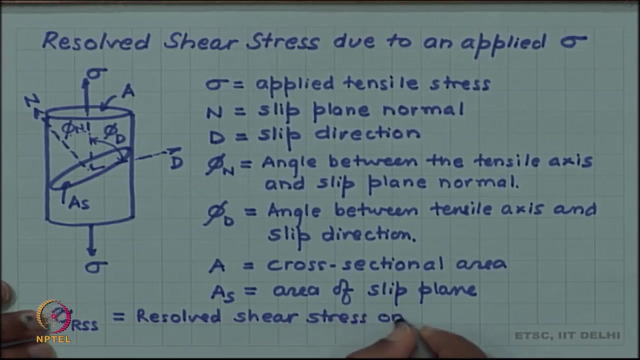 And A? s is the area of slip plane. So with these variables we can now try to find what is the resolved shear stress. So tow R s s. This is a resolved shear stress on the slip plane, in the slip direction. So tow R s s. is 1,, 2,, 3,, 4,, 5,, 6,, 7,, 8,, 9,, 10,, 12,, 13,, 14,, 15,, 16,, 17,, 18,, 19,, 20,, 21,, 22,, 23,, 23,, 24,, 24,, 25,. 25,, 26,, 28,, 24,, 26,, 27,, 28,, 29,, 30,, 29,, 31,, 32,, 33,, 33,, 33,, 34,, 35,, 37,, 38,, 38,, 39,, 39,, 40,, 40,. 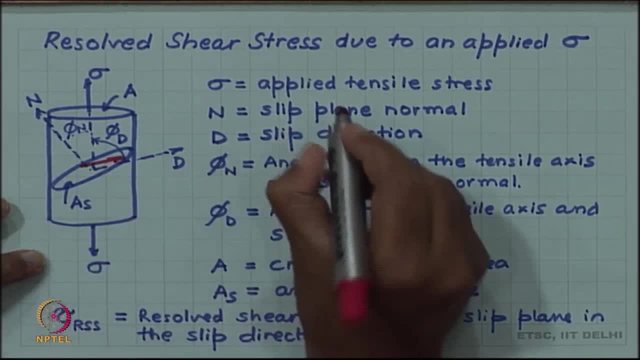 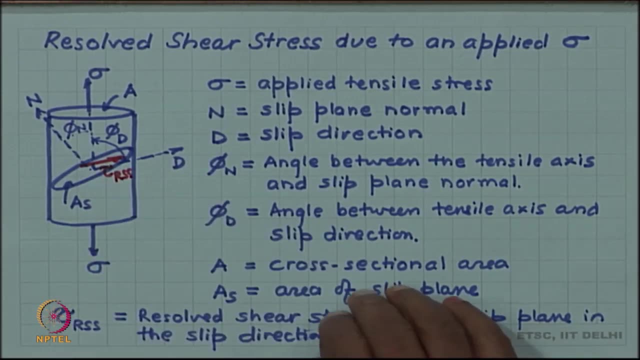 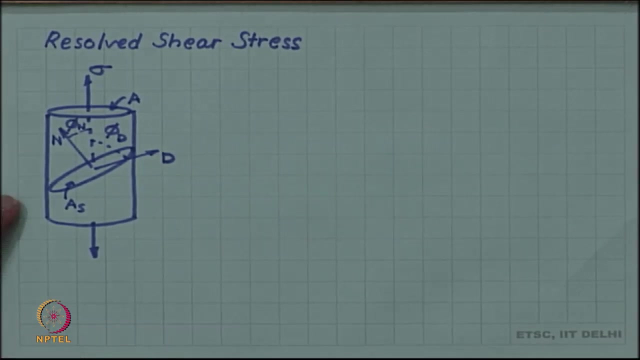 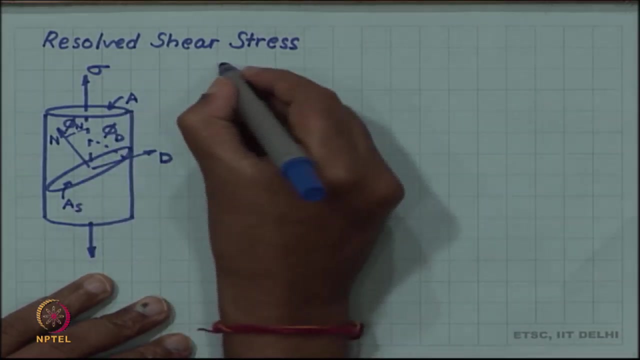 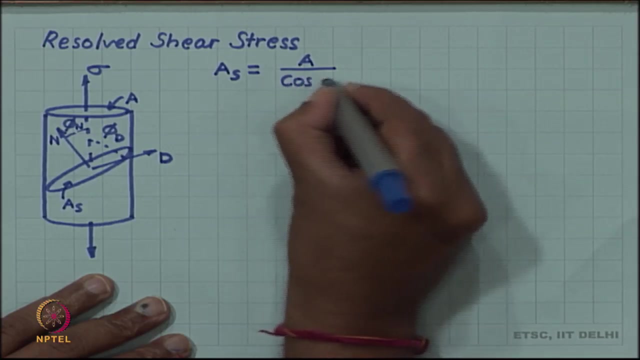 on this plane, acting in that direction. So what is the value of this tow RSS in terms of these variables? So first of all let us relate A and A S so geometrically we can show the slip plane area A. S will be the cross sectional area A divided by cos phi n. Also, 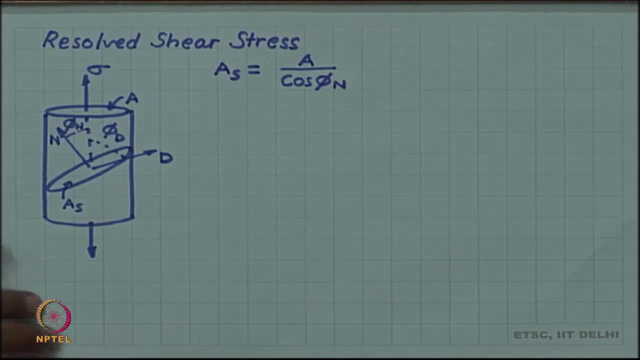 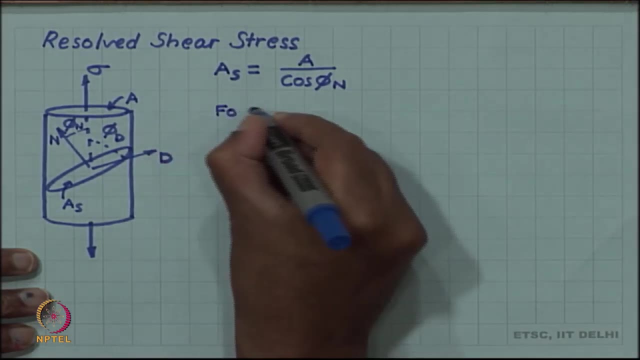 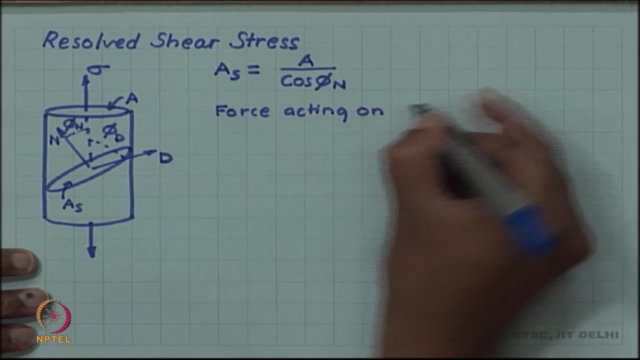 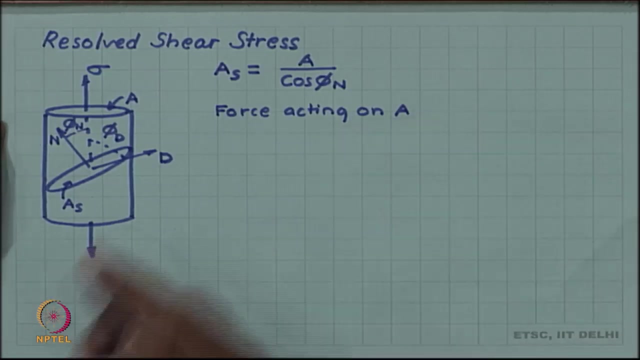 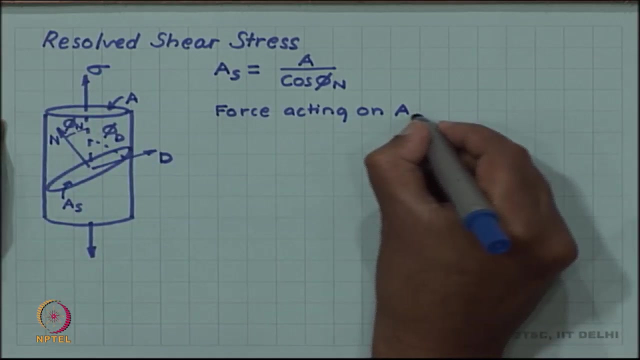 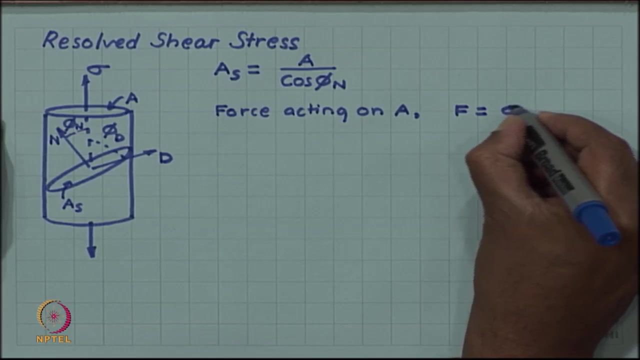 let us try to find how much force is acting on this cross sectional area. So tensile force acting on A. so this, by definition, since the definition of a stress itself is force divided by cross sectional area, So this force will be given by F- is equal to this stress times. 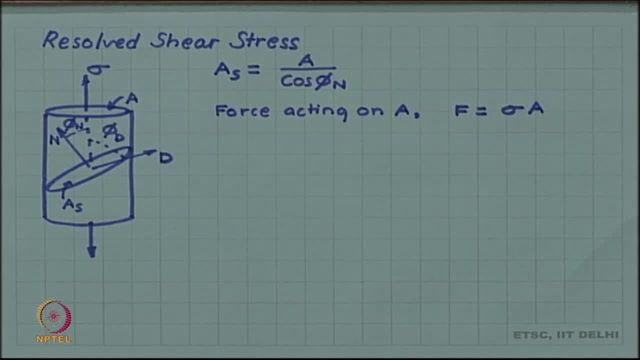 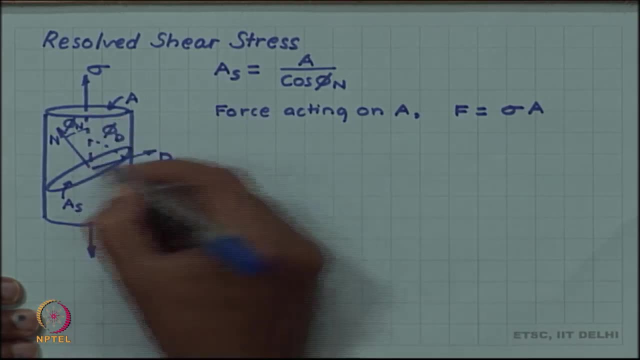 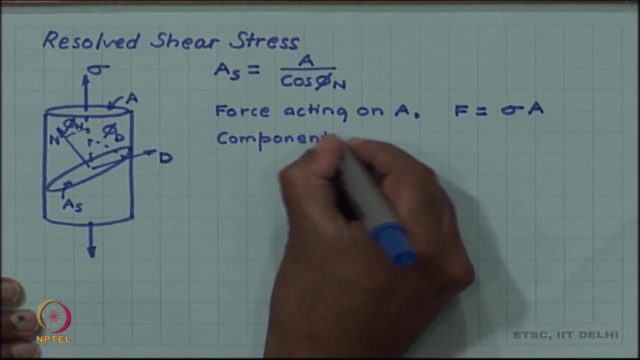 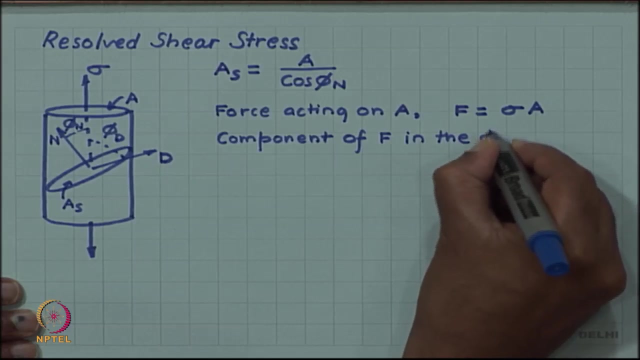 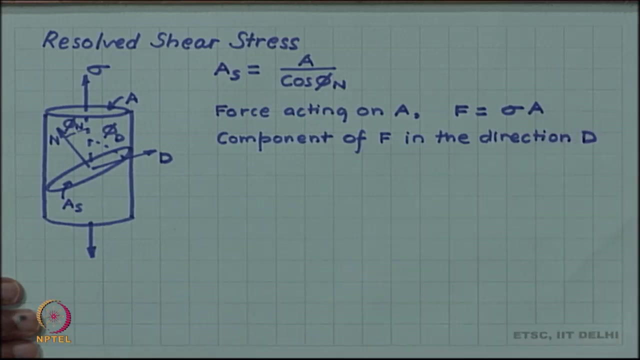 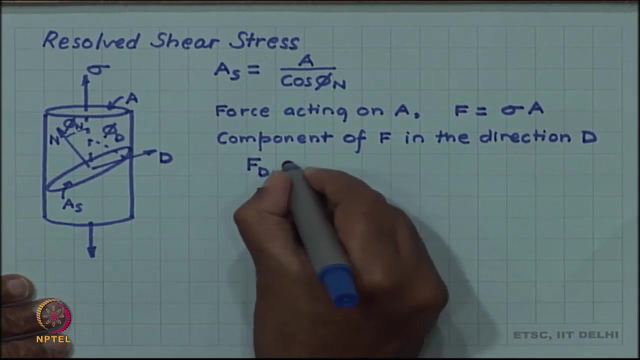 A, because this stress is Force divided by area. so force acting on A is F A. Let us take the component of this force in the direction D, component of F in the direction D, that is, in the slip direction. So let us call that component F D. So this will be simply F cos phi d, because phi d recall. 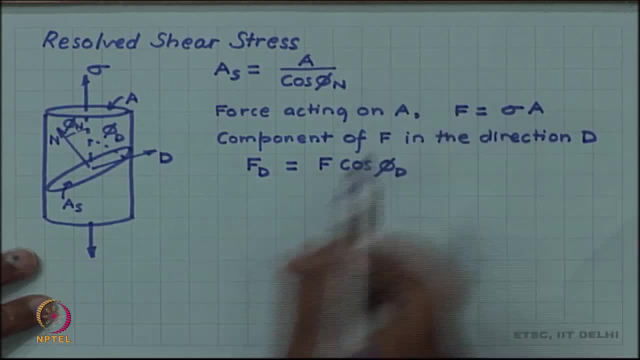 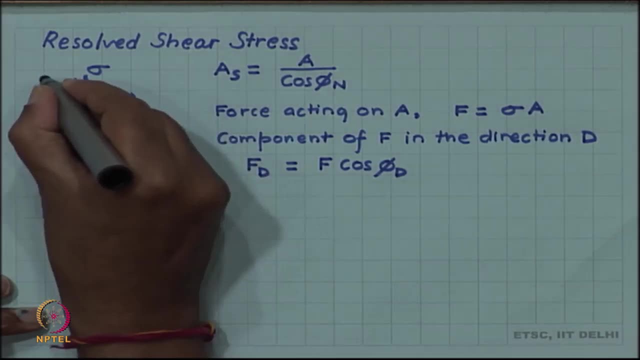 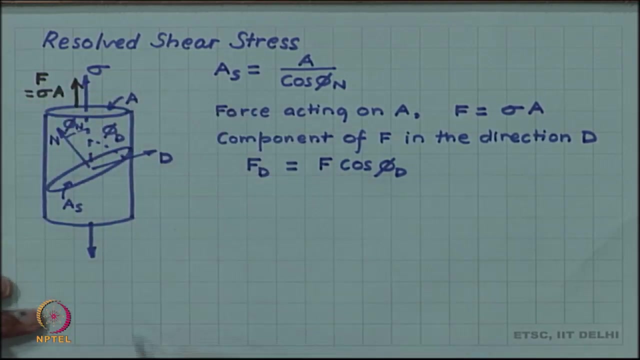 that this tensile force will also be acting in the same direction as the stress. So this force acting on this force- F is equal to sigma a- is acting in the same direction. So it makes an angle phi d with the direction d and we know that to take the component of any given force, we 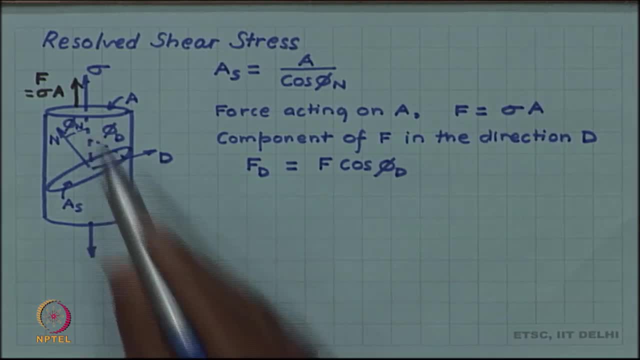 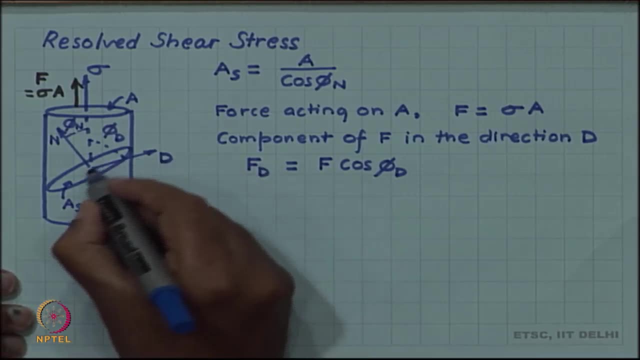 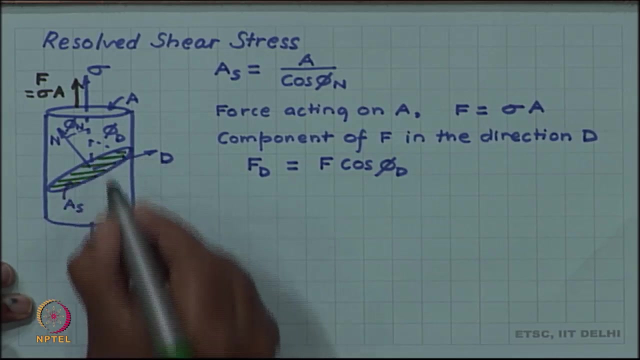 multiplied by cosine of the angle between the direction and the force. So F d is F cos phi d. now this F d is what will generate the shear stress. So if we now think of this F d acting on the slip plane a s, so the plane on which it is acting is a slip plane a s. 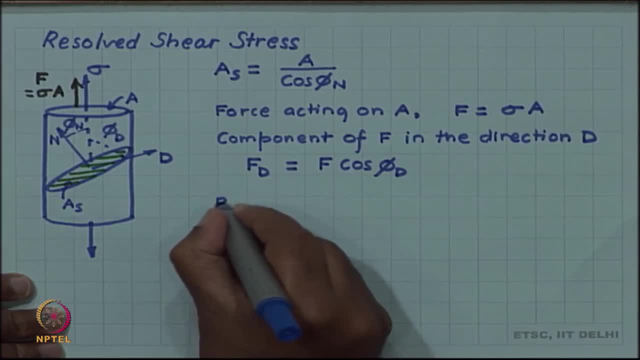 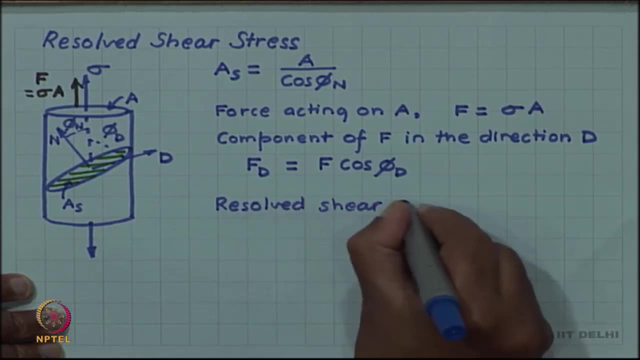 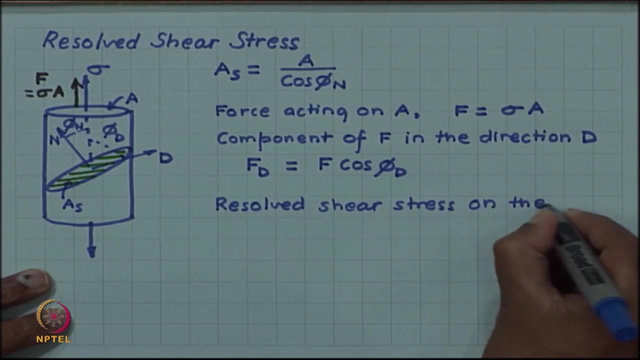 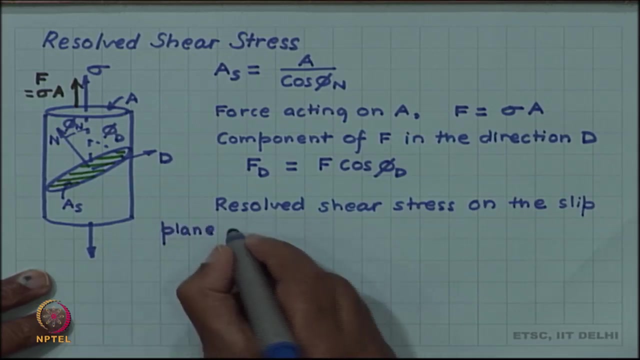 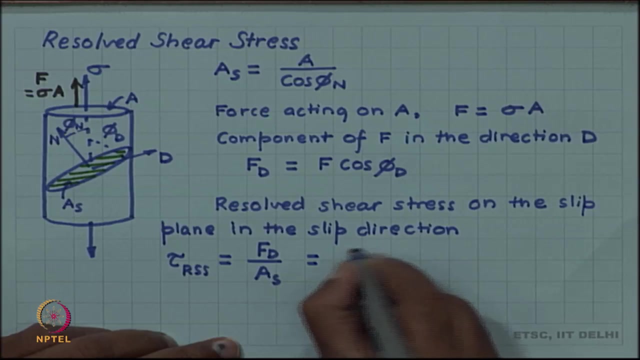 So the shear stress resolved, shear stress, plane on the slip plane, in the slip direction, rho r s s will be. the force is F? d and it is acting on an area, A? s. So F? d we have already found as F cos phi d and A? s we have found as A by rho r. 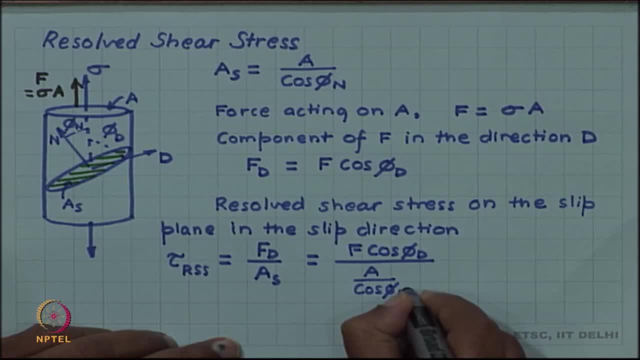 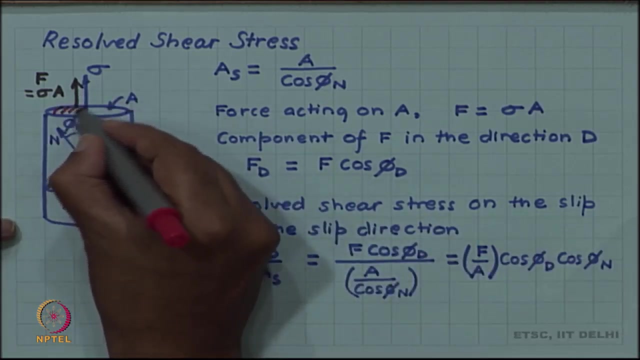 by cos phi n. So we can see that we can write this as F by A, cos phi d cos phi n. but note this: F by A. F is acting. F is acting on the cross sectional area and we are dividing it by the area cross sectional. 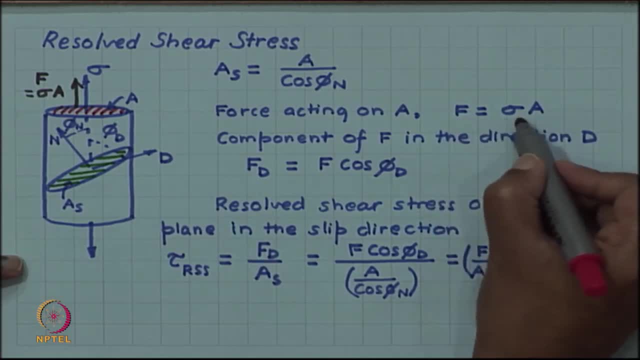 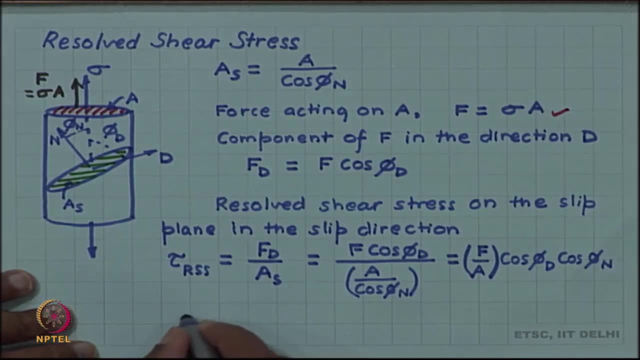 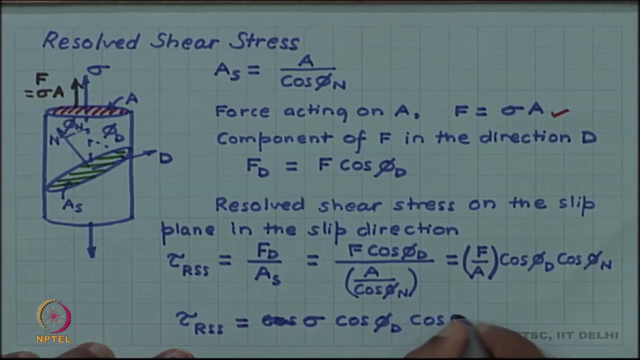 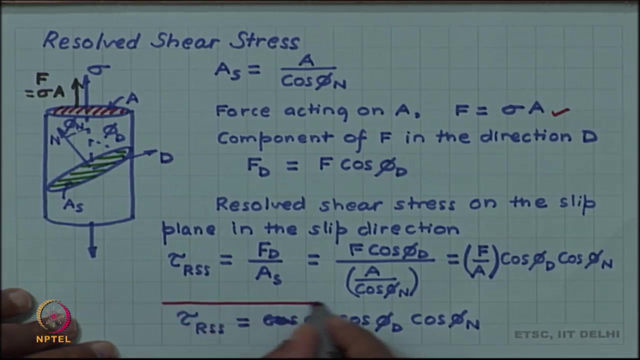 area. look at this relationship. So F by A is simply F by A is sigma, the applied stress sigma. So we then get our final relationship, which we will be using- sorry, we will be using this- So this becomes our resolved shear stress. So we see the resolve shear stress depends. 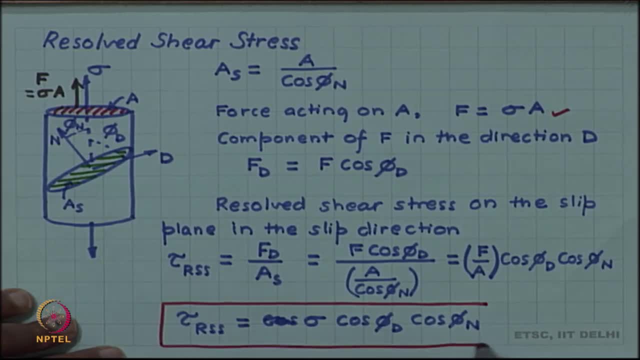 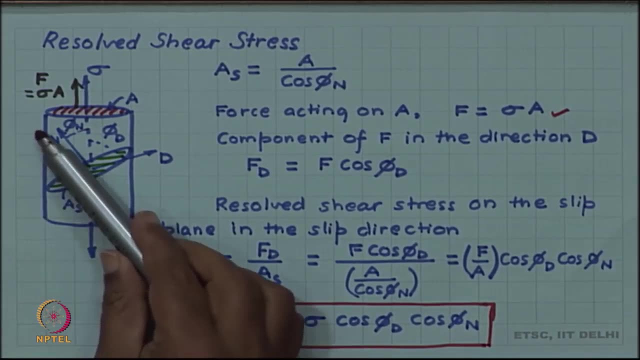 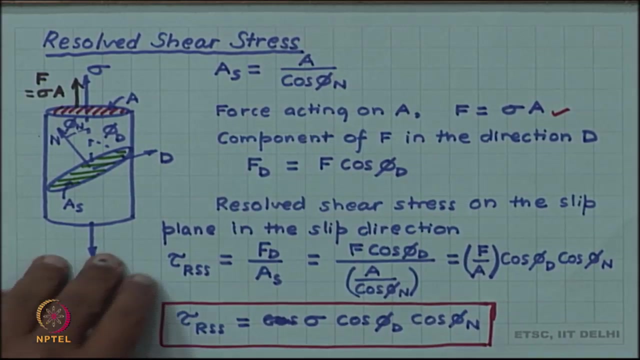 not only on the applied stress, but also on the orientation of your slip system: orientation of the slip plane normal and the slip direction cos phi d, cos phi n. So we have established this relationship which we wanted for the resolved shear stress. Let us look at some of the consequences of 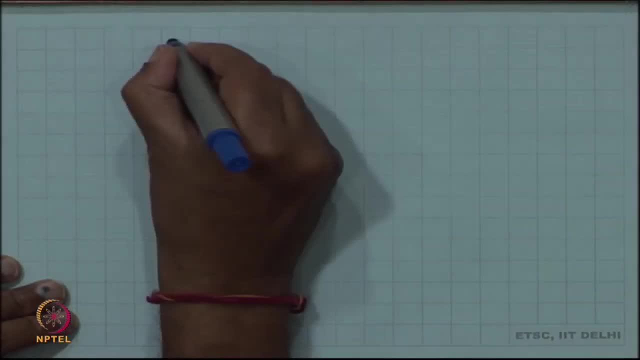 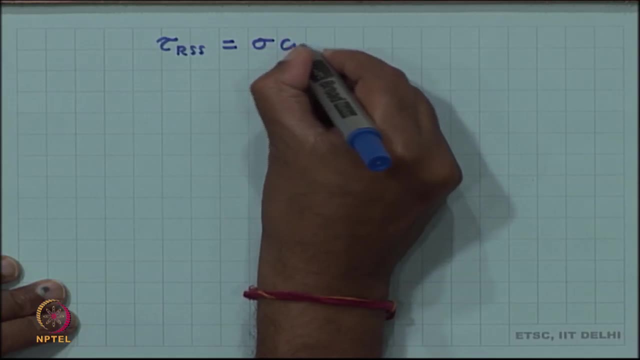 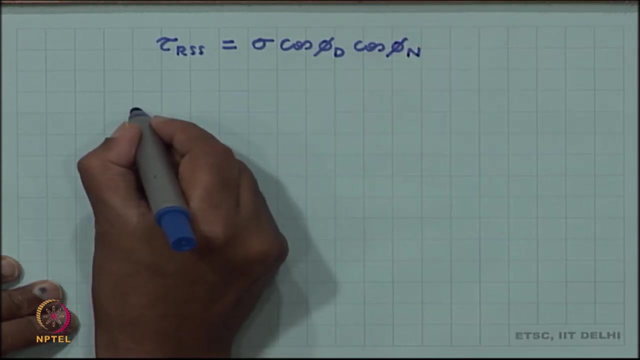 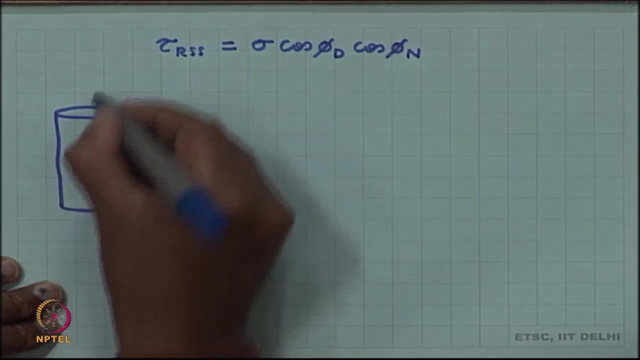 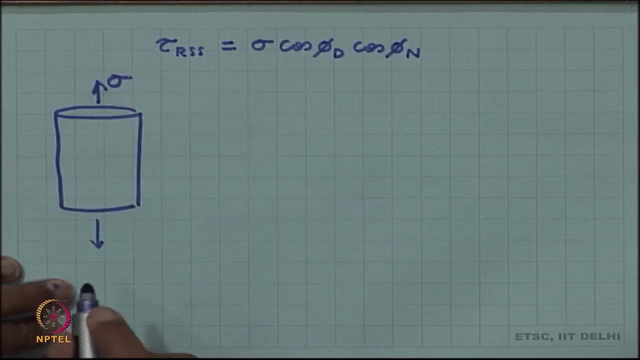 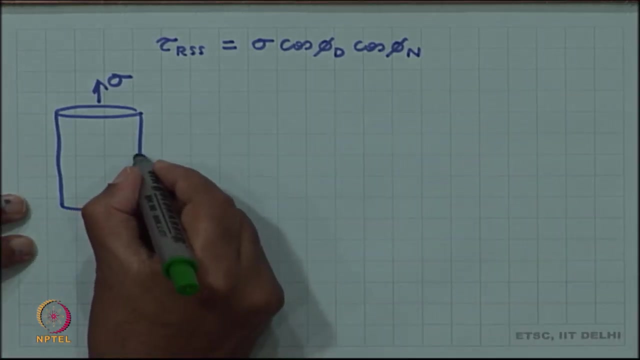 this relationship. So we have tau: RSS is equal to sigma, cos phi d, cos phi n, and this is our sample. So this is our sample. Now consider a plane which is normal to the stress axis. So for this, the slip plane, normal. 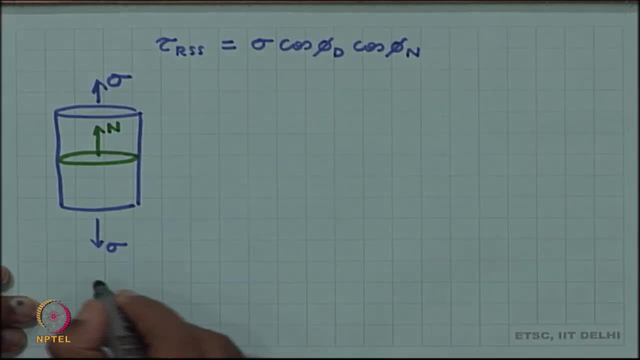 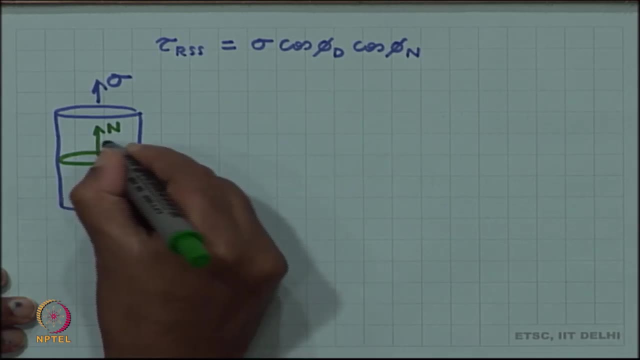 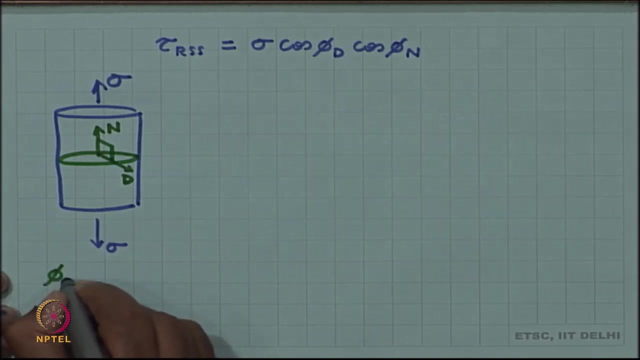 is in the stress axis, So, which means the slip direction. any slip direction which you will take will always make an angle 90 degree with the stress axis. So phi d for this case, phi d will be 90 degree, and so resolved shear stress will be 0.. So no resolved shear stress. 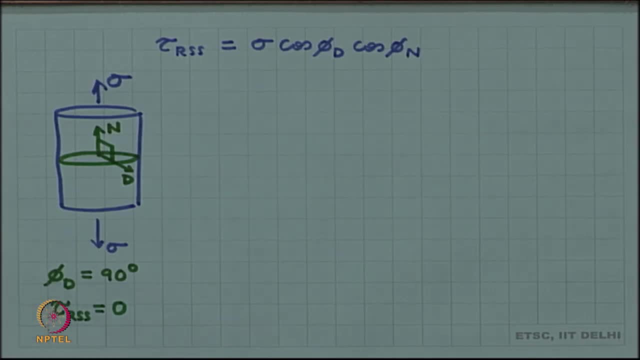 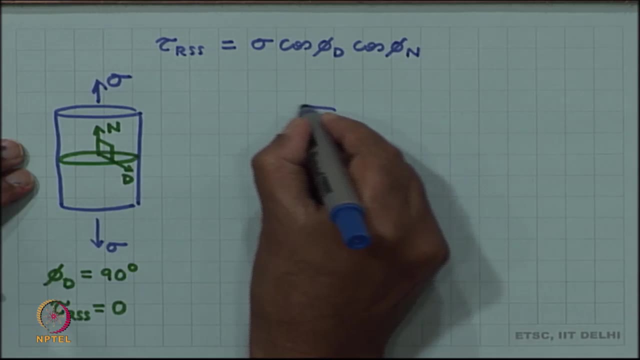 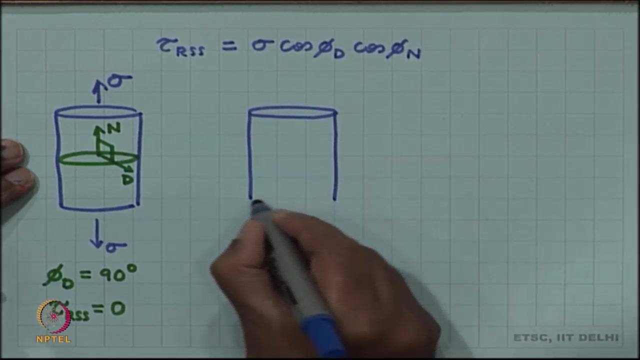 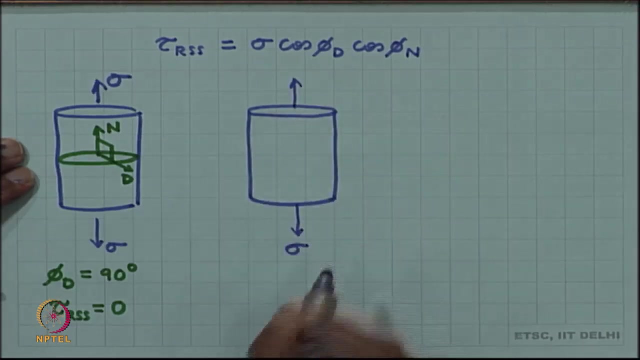 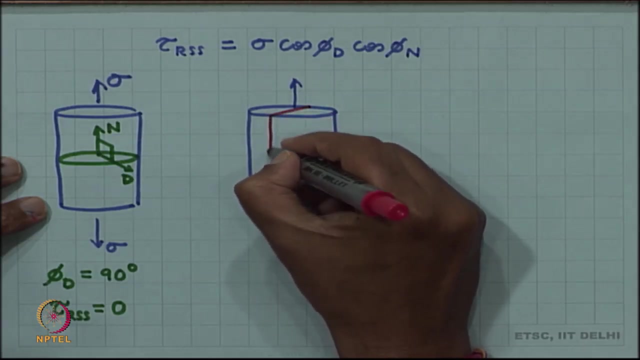 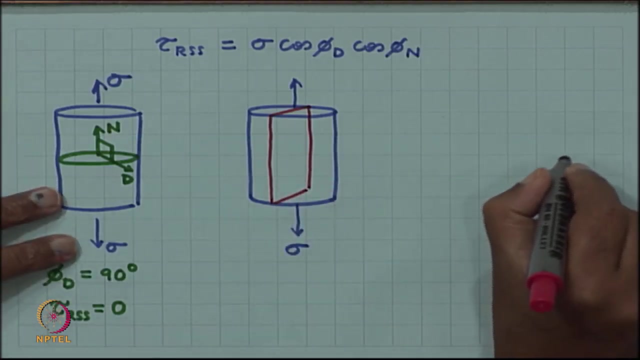 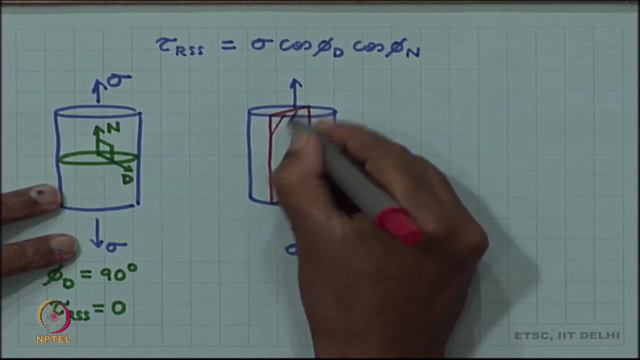 can exist on a plane which is perpendicular to the stress axis. Now let us consider another case in which I now take a plane which is parallel to the stress axis. If I take a plane like this, you can. you can see that the plane normal. 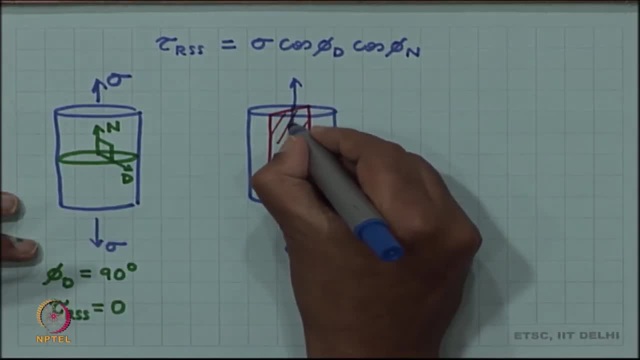 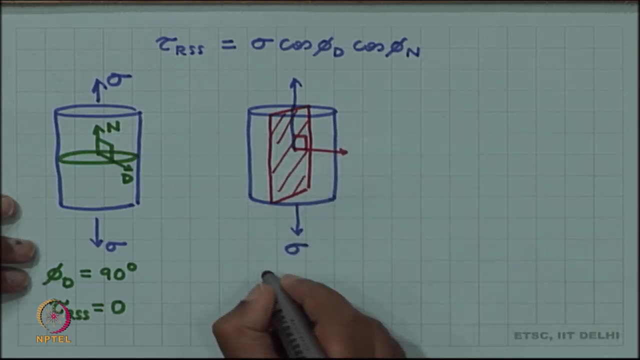 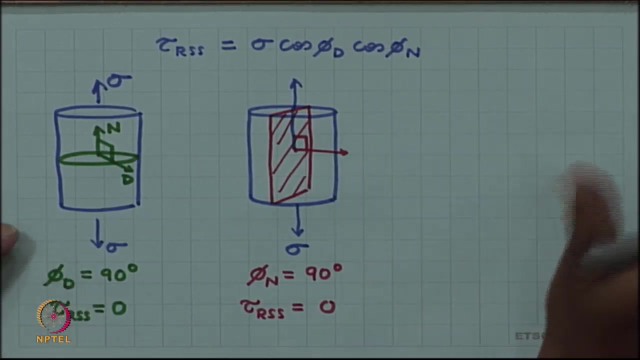 will make an angle 90 degree with a stress axis. So now phi n, Irrespective of phi d, phi n will be 90 degree and tau RSS will again be 0. So we find that there will be no. in fact, these are the only two planes for which the resolved shear stress. 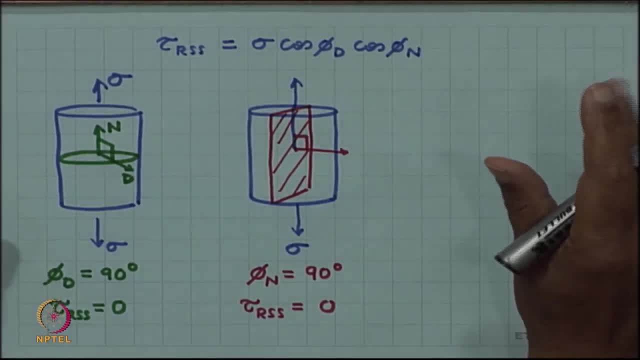 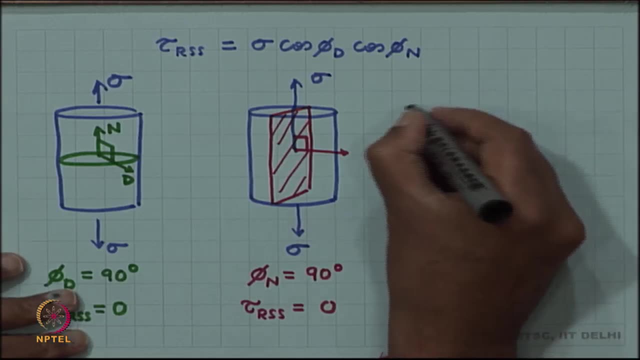 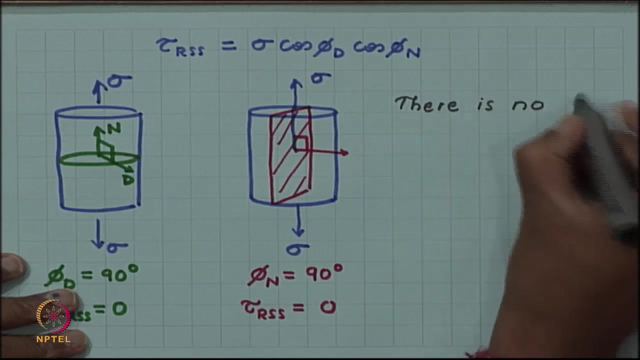 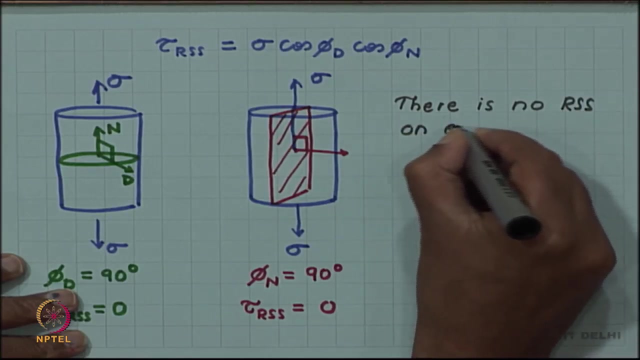 has to be 0. All other inclined planes, they will be some resolved shear stress. So we let us note down this that there is no resolved shear stress. there is no RSS on a plane either. perpendicular.